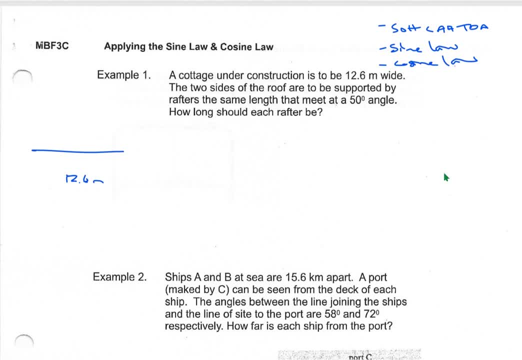 And then it says the two sides of the roof are to be supported by rafters that are the same length and that meet at a 50 degree angle. So I'm going to draw this triangular roof- And these things over here are called rafters- And I'm going to make those little markings. 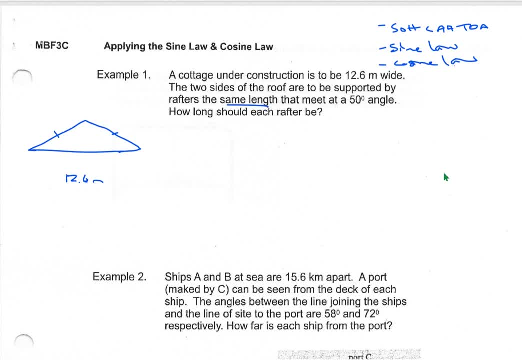 that show that they're the same length. It's the same length, And these two rafters meet at an angle of 50 degrees. How long should each rafter be? So they're asking for this length over here, Okay, or this length of the other. the other one's exactly the same, So we're looking at what's. 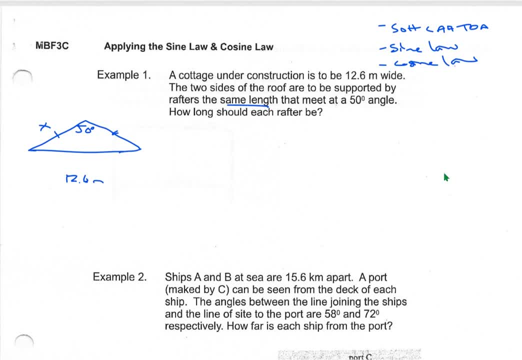 what is given to us. we have one side, one angle, which is nice for the sine law, But we're going to need more information because even for the sine law we're going to need one more angle. So we could say: sine, 50 degrees over 12.6 equals sine. And then we're going. 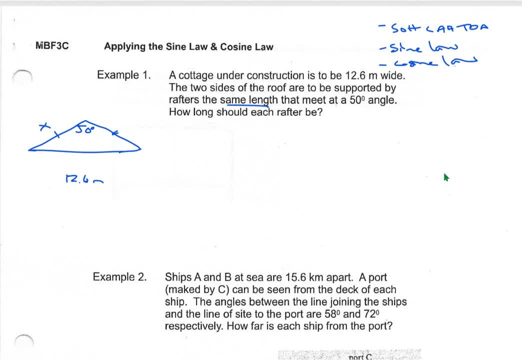 to have one more angle over x, And we don't have it right now. So what we need to know is that this is an isosceles triangle. you see, those two sides are equal. I saw, I saw salis triangle. So when the two sides are equal, it means that these two angles will. 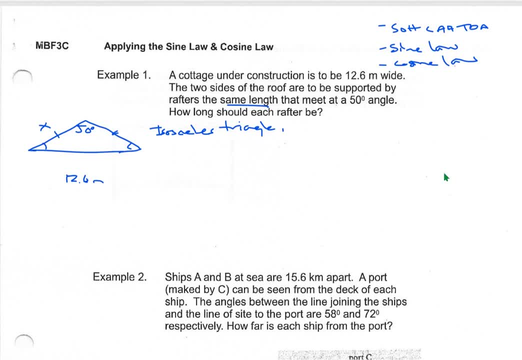 also be equal. So since all of the angles add up to 180 degrees, then 50 degrees plus the angle on the left plus the angle on the right, but they're the same. Okay, so we're going to have one more angle over x, And we don't have it right now. So 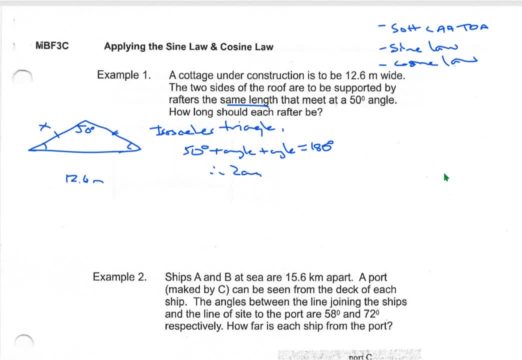 what we need to know is that this is an isosceles triangle. You see, those two sides are equal, And we don't have it right now. So what we need to know is that these two angles are equal. Okay, so now we have 60 degrees andesque. This is an isosceles triangle, Since those 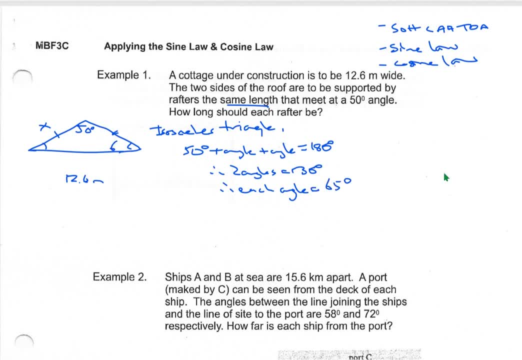 two angles add up to 180 degrees. therefore, the two angles add up to 180 minus 50, so 130 degrees. therefore, each angle is half of that which is 65 degrees. So I know that this here, okay. so sine 50 degrees divided by 12.6 equals sine 65 degrees divided by x. and then you cross. 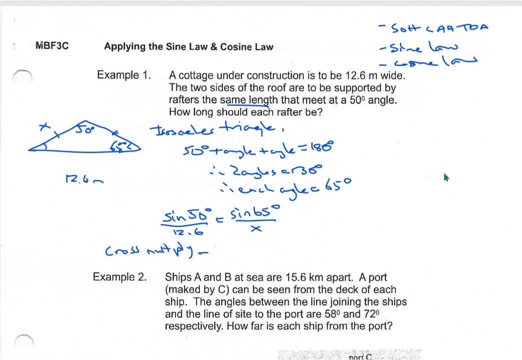 multiply, and you just refer to how to use the sine law. if you forgot, uh, you have to go back in and watch the videos and do some practice. so i'm just gonna, i'm gonna skip all the steps just because i don't have much paper, much paper here, but i'm going to leave it to you to, um, figure out. 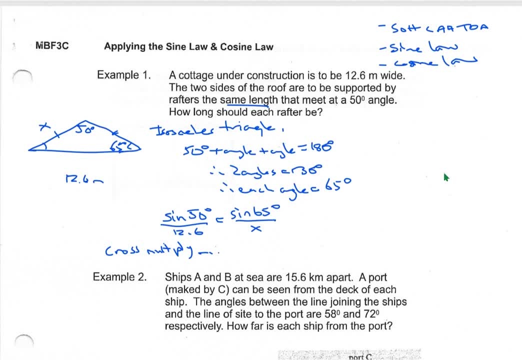 the sine law from before. okay, and it turns out to be 14.9. okay, so x equals 14.9 and it's meters, okay. or we could do this a different way. we could say: because it's a right angle triangle. i'm sorry, it's not a right angle triangle, because it's isosceles. 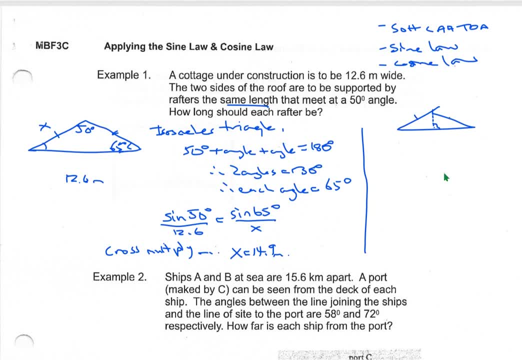 and in an isosceles triangle, if we make the height, it actually cuts the base in half. so this would be: the total is 12.6. so this is 6.3, and this is 6.3, and it also will cut this angle in half. so instead of 50 degrees, it's 25 and 25, so we end up with a right angle triangle. 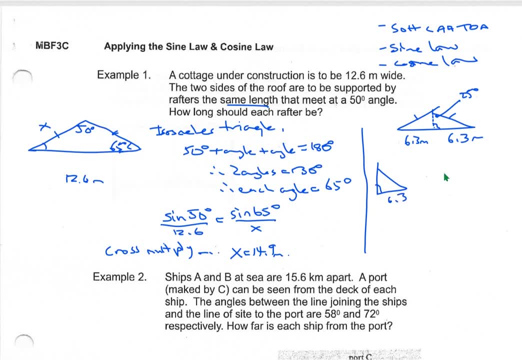 anyway, we take half of it is a right angle triangle, so this is 6.3 and in here is 25 degrees and we're trying to find x. so from the 25 degrees i have my opposite and i have my hypotenuse. so opposite and hypotenuse, that would be up here. 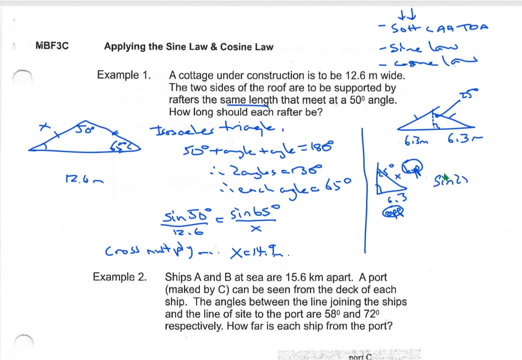 sine. so sine of 25 degrees equals opposite, which is 6.3 over hypotenuse. press multiply i get x sine 25 degrees and i have my hypotenuse. so i have my hypotenuse 2 over my hypotenuse right and this thing over here. as i said했 this, i'll just look. 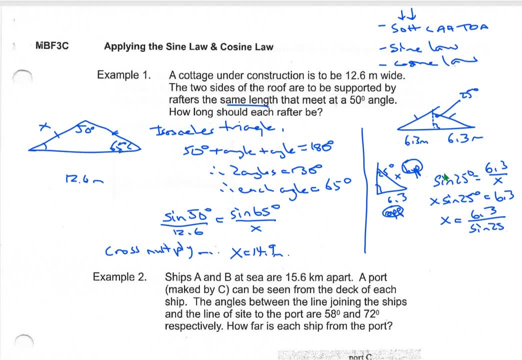 at the equation of the hypotenuse as this. it goes back in my calculator and then i'll find the particle sickness angle. so that's its right angle. so this is x and around 25 degrees. so i almost had two sides representing the same vertical axis. 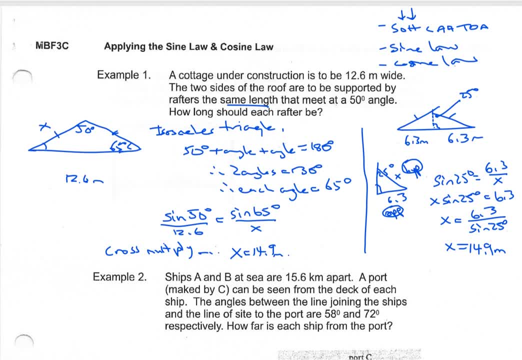 minute right, and so what's going to happen? i'm going to have to find over here the right angle, and it comes back in front right, and the stuff that i've done to this is its negative angle, and it gets ruined. but whatever, that's fine. so then what's going to happen is that: 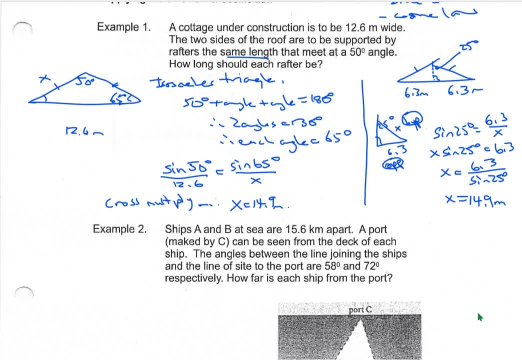 i well, that's a one part of this has two parts to it, so i'm going to turn it upside down. Of course, we finish with the therefore statement. Therefore, the rafter should be 14.9 meters long. All right, let's do another one. 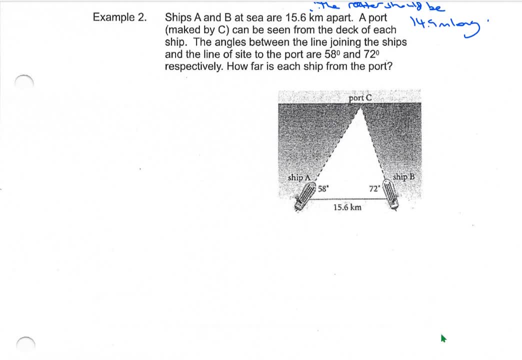 Ships A and B at C are 15.6 meters apart, So this one's nice because they actually give us a diagram So it's easier. A port marked by C- This actually got some spelling mistakes in here, So marked can be seen from the deck of each ship. 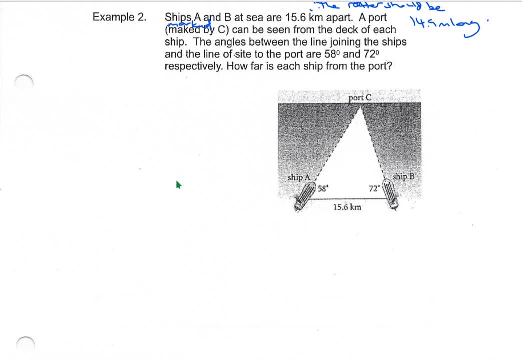 The angles between the line joining the ships and the line of sight S-I-G-H-T to the port are 58 degrees and 72 degrees respectively. How far is each ship from the port? So what they're asking for, if this is A ship A is here, then this is little A. 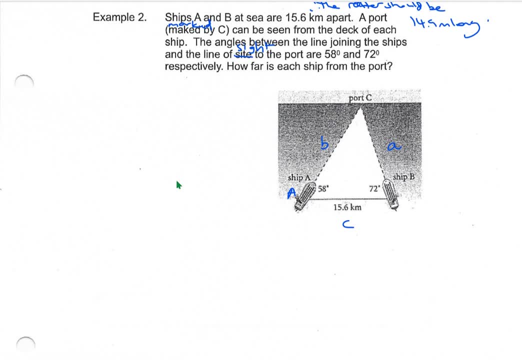 Ship B is on this side, so this is little B, And then here we have our C. So if we want to solve for little A, then I could use the sign law And I could say: ship A or sign of big A divided by little A equals something else. 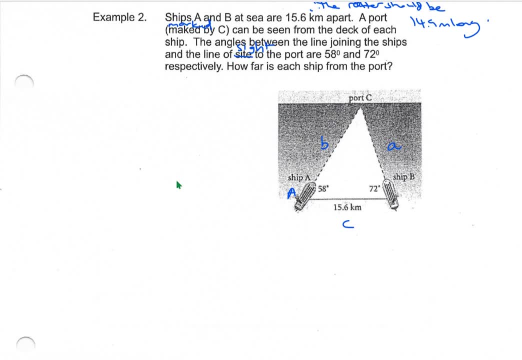 And so for the something else I'm going to need: an angle and a side given to me. And with the Bs, I have the angle, but I don't have the side across. And with the Cs, I have, I don't have the side across, but I don't have the angle. 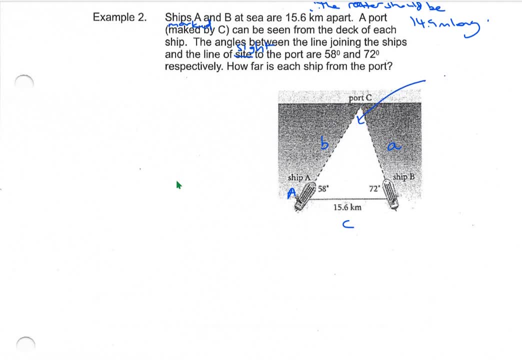 So here what we could do is we could calculate this angle C. So angle C is equal to 180 minus 58 minus 72. So 180 minus 58 minus 72 is 50 degrees. So now that I have angle C is 50 degrees, I can use the sign law because I have these pairs. 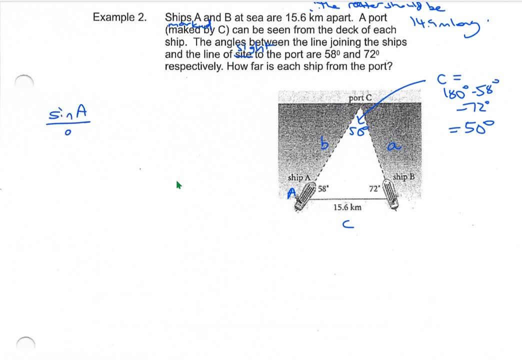 So I can say: sine Big A over little A equals sine big C over little C, And so sine 58 degrees over little A equals sine 50 degrees over 15.6.. And cross multiply A sine 50 degrees equals 15.6 sine 58 degrees. 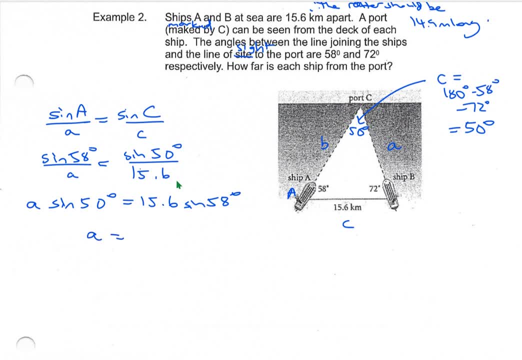 Divide both sides by sine 50 to get A alone, And I get A is 15.. 15.6 sine 58 degrees over sine 50 degrees. Into my calculator this thing goes all at once: 15.6 sine 58 divided by sine 50.. 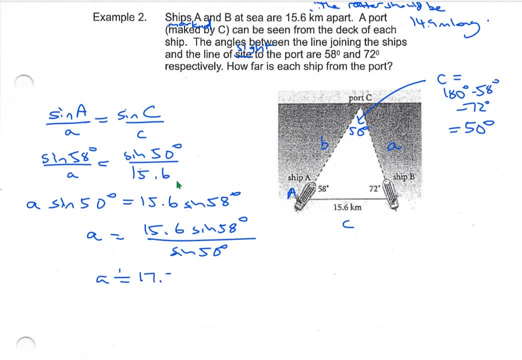 17.3.. So A is approximately 17.3 kilometers And if you look at the diagram that looks reasonable. 17 looks reasonable there. And then do the same for side little b. Okay, so that's using the sine law. 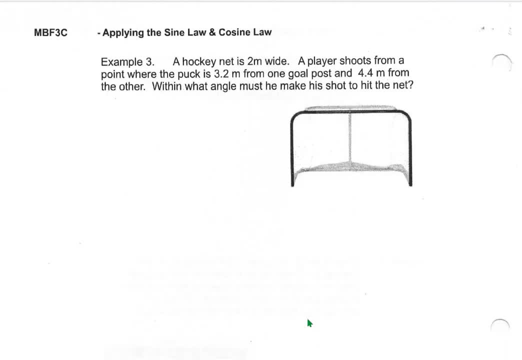 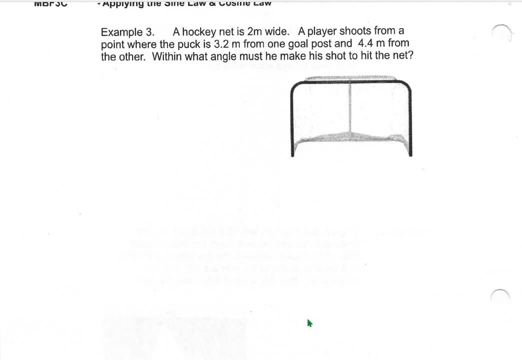 So every question is different depending on what information you get. Last one: A hockey net is two meters wide. A player shoots from a point where the puck is 3.2 meters from one goalpost and 4.4 meters from the other. 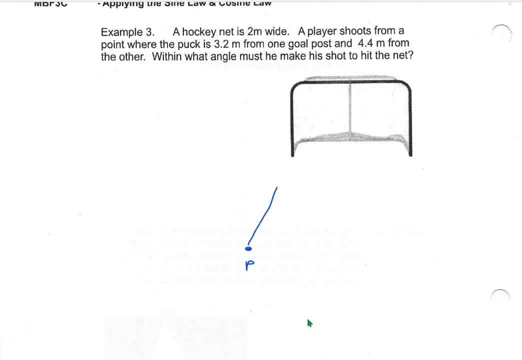 So let's say my puck is over here And this is 3.2.. 2 meters from one goalpost and 4.4 meters from the other goalpost. Within what angle must he make his shot to hit the net? So he needs to make his shot within this angle over here. angle P. 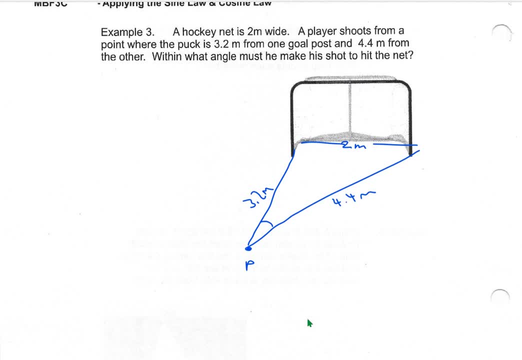 We're also given that the net is 2 meters wide. So here's our triangle. Now I don't have any angles given. If I don't have any angles given, then I must use the cosine law, Because I don't have a pair of an angle and a side given to me. 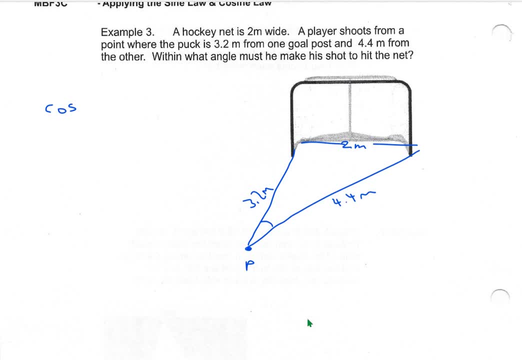 So we'll use the flavor of the cosine law that starts with the angle with the capital letter. All right, so let's call these guys Q and R, And so this is little r, this is little q and this is little p. 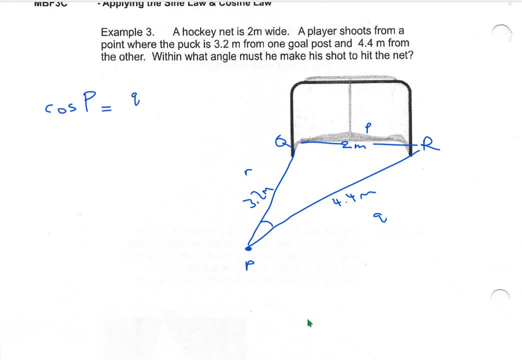 So cosine of big P is equal to little q squared plus little r squared minus little p squared over 2.. Little q, little r. So putting all the numbers in cosine P equals 4.4 squared plus 3.2, squared minus 2, squared over 2 times 4.4, times 3.2..